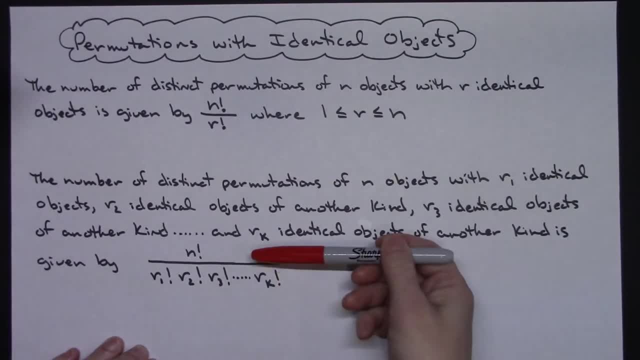 objects of another kind. And that formula is going to be given by n factorial. over all of those different factorials multiplied So r sub 1 factorial times, r sub 2 factorial, r sub 3 factorial times, however many, you would have r sub k factorial. 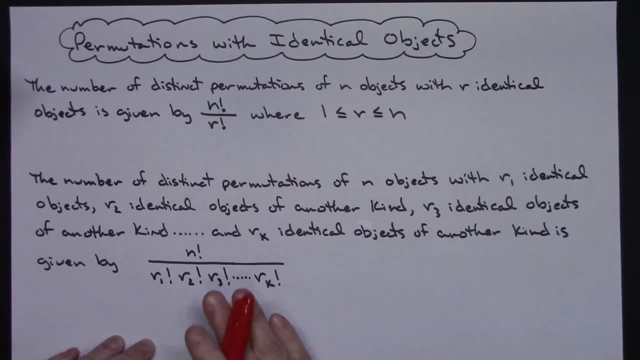 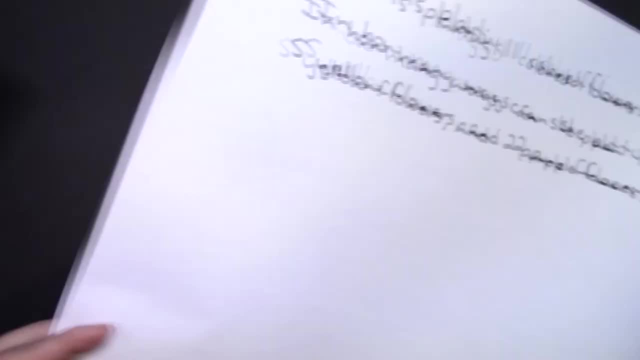 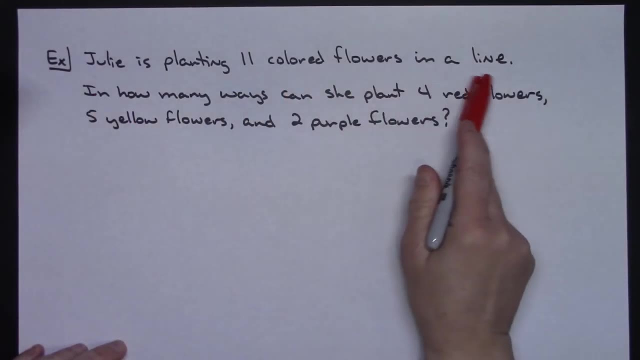 Alright, So two different formulas here that we're going to be focusing on. My example is going to focus on this second one. but permutations with identical objects? Now what an example of that might look like. Let's say, Julie is planting 11 colored flowers in a row. 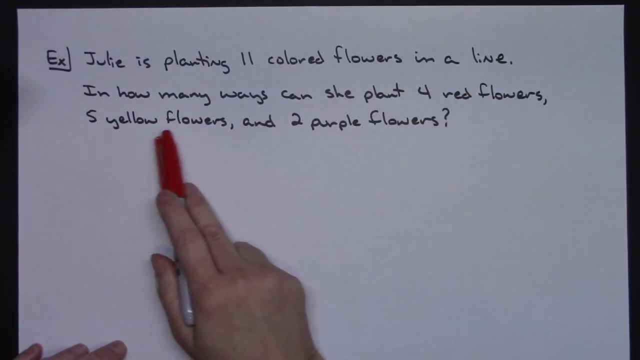 In how many ways can she plant 4 red flowers, 5 yellow flowers and 2 purple flowers? So we've got identical objects, flowers, but they're just of a different kind Because they're of a different color. Alright, 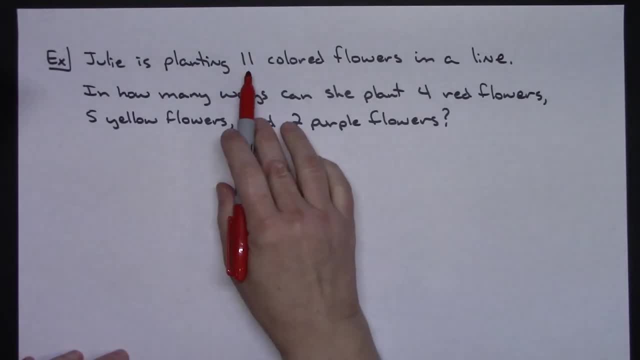 So we're going to set this up using the second formula. I've got a total of 11 flowers, So that was going to be my 11 factorial on top. Alright, Now I'm going to take each one of those 3 different colored flowers. 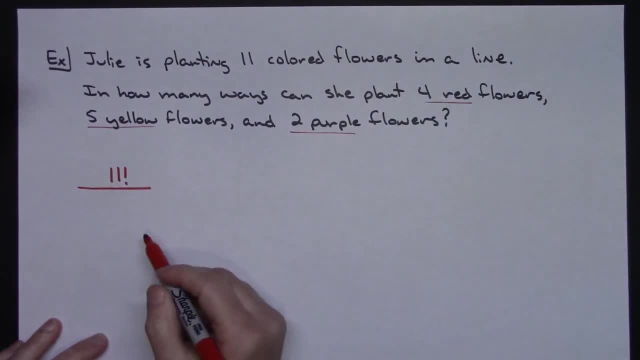 So I've got 4 red, I've got 5 yellow and I've got 2 purple. Alright, So I need a 4 factorial times a 5 factorial Alright. So I've got 4 red, I've got 5 yellow and I've got 2 purple. 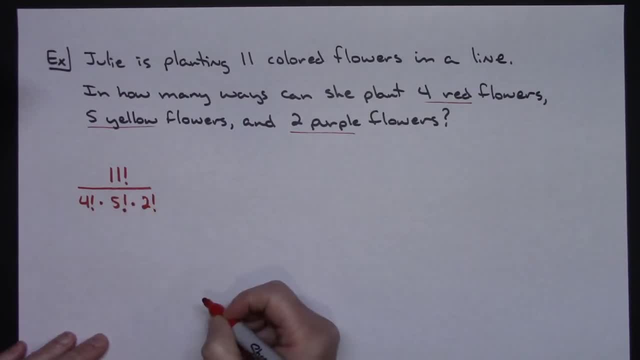 Alright. So I need a 4 factorial times 2 factorial on the bottom. Alright, Now let's do some simplifying with this, As opposed to just grabbing a calculator right away. Let's go ahead and take that 11 factorial down to 5.. 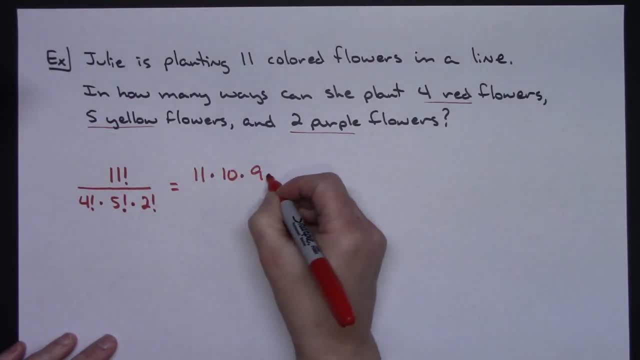 So 11 times 10 times, 9 times, 8 times, 7 times 6 times 5.. And then we're going to leave that as a factorial And then we've got 4 factorial times, 8. times our 5 factorial times the 2 factorial on the bottom. 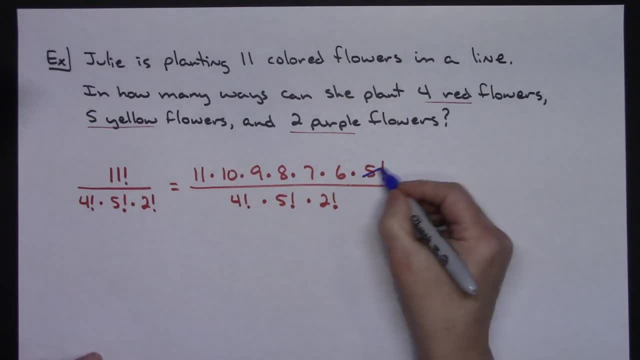 All right, that's going to allow me, then, to cross out the 5 factorials, really simply there. All right, now let's go ahead and break down the denominator there a little bit: 11 times, 10 times, 9 times, 8 times, 7 times 6 across the top. 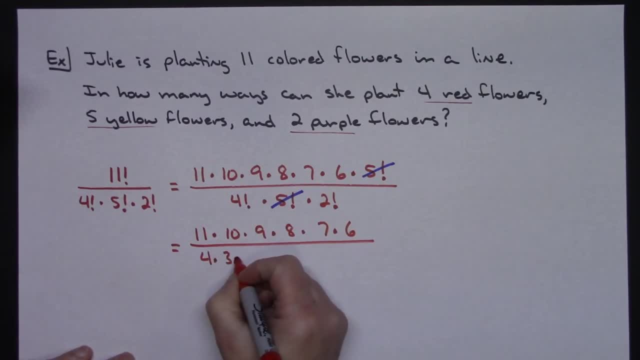 And the 4 factorial is going to be a 4 times 3 times 2 times 1.. And the 2 factorial then will be the 2 times 1.. All right, so let's do some crossing out here. Let's do 4 times 2 is going to give me the 8 on top so I can cross all of those out. 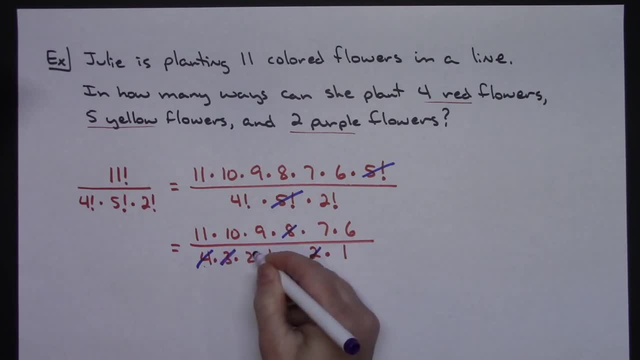 And 3 times 2 is going to give me 6, so I can cross all 3 of those out as well. All right, getting this down to a pretty small number now. So now we've got just a 1 on the bottom. 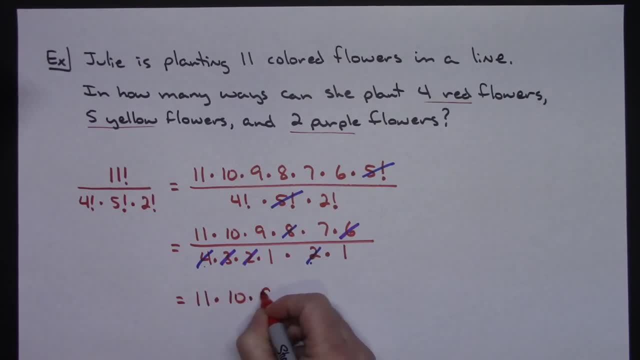 Across my top. I've got an 11 times 10 times 9.. 9 times 7 and that's going to be a total of 6,930.. So there's 6,930 ways that Julie can plant the flowers in a line. 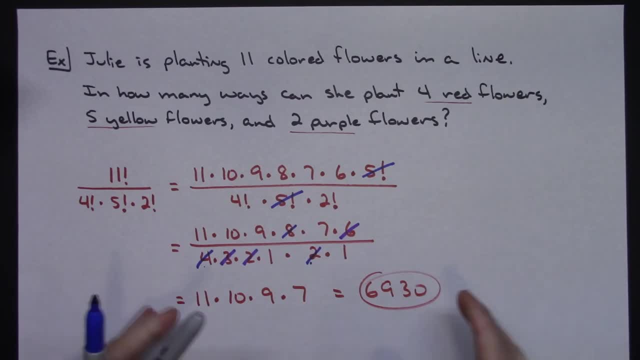 Okay, so just one quick example there with a couple formulas on how you work out permutations with identical objects. Definitely thanks for watching, Really appreciate it. Give me a thumbs up and be sure and share with your friends. Thanks. 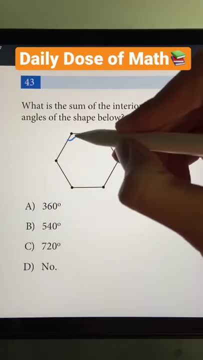 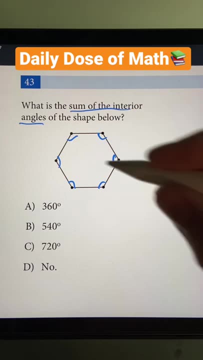 What is the sum of the interior angles of the shape below? So all of the interior angles are just going to be the angles inside the shape, And it's actually really easy to find the sum of the interior angles because it follows this one formula, which is 180 degrees times n minus 2,. 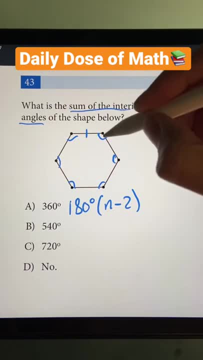 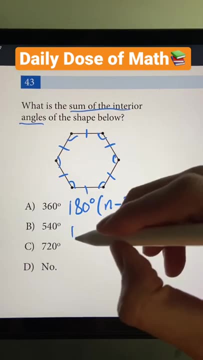 where n is the number of sides of the shape. So let's count that. So we have 1, 2, 3, 4,, 5,, 6.. This is a hexagon, which means we plug 6 in for n right here. So 180 times 6 minus 2,.